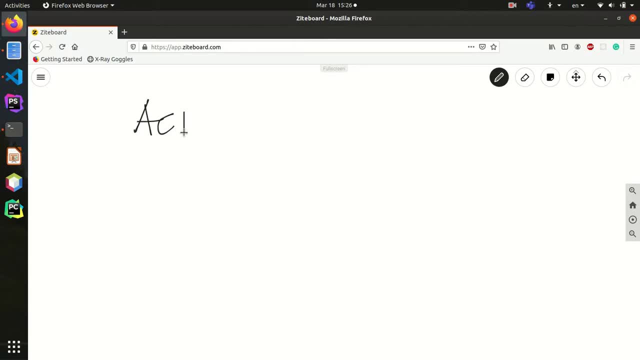 name here Ackermann function- is a recursive function. So the recursive function means that it calls itself repeatedly. So the Ackermann function, let's say that we have function a, m, n. it's going to return us three outputs. So 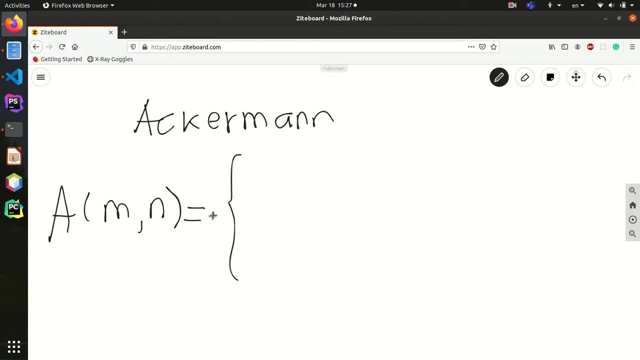 three types of output. actually, In case m is zero, it's gonna return us n plus 1.. In case m zero, okay. in case n is zero, it's gonna return us a m minus one and one. in case n is zero. and in case neither m nor n is zero, then it's gonna return us a m minus. 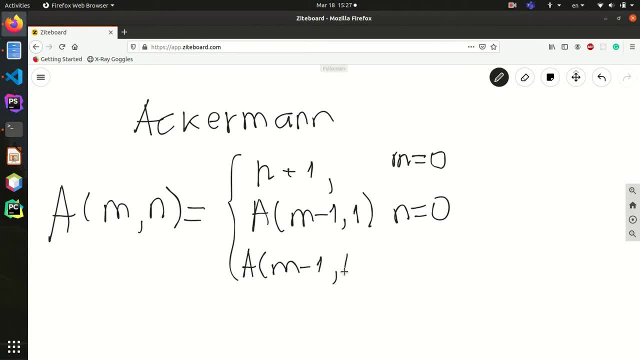 one, and then a, m, n minus one. okay, in case m and n is greater than zero, n is greater than zero and n is greater than zero. all right, let's see how this function actually works. so let's begin with a simple explanation. let's start with a simple explanation. let's start with a simple explanation. 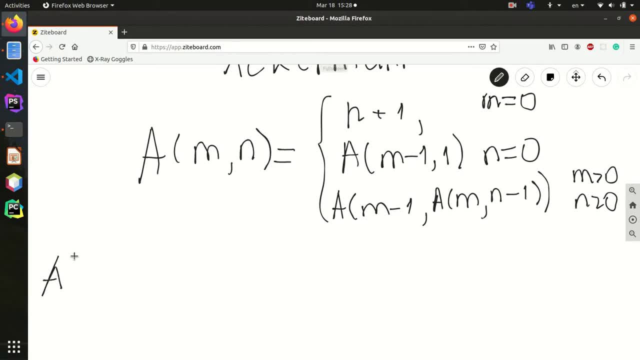 let's begin with. let's say a, m is 0 and n is 5. so in this case our function is going to return us m plus 1, because m is equal to 0. so it's gonna return us m plus 1 of n plus 1, which is 5 plus 1 and 6. and let's have a look another example. 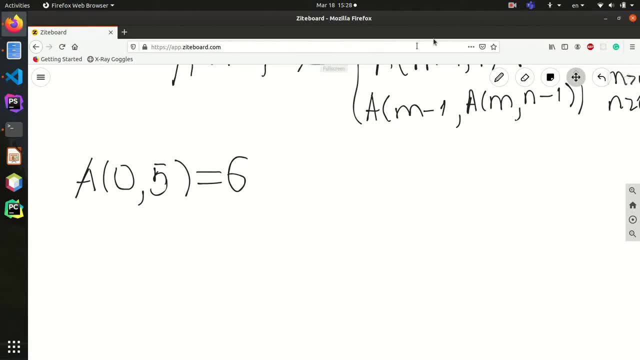 a bit complicated. let's say: let's say that we have a 1 and 2, so in this case neither m nor n is zero. so let's say that we have a 1 and 2, so in this case neither m nor n is zero. so 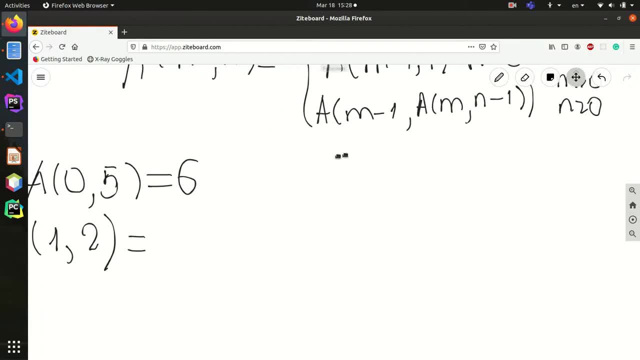 we're gonna come here and the function is gonna call itself like this: a, M minus one, which is one minus one zero, and a again m and m is equal to zero here. so who help me? help me, Don't forget: m is 1, still here, m 1, and n minus 1, which is 2 minus 1, 1.. 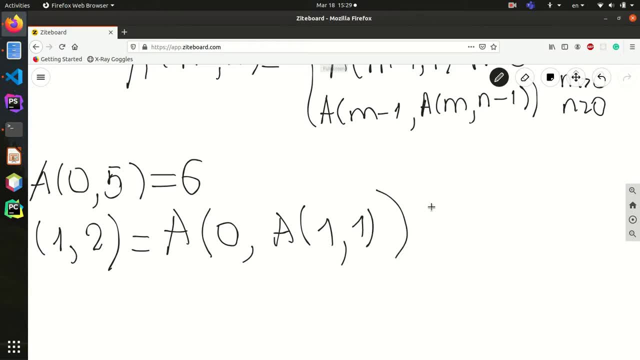 So here things got a bit complicated, because here inside of an anchorman function I have one more anchorman function here. So I'm going to calculate it separately and then I'm going to come here and write its output again. So I'm going to calculate this part. So this a11 again meets this condition. so I'm going to do: a11 is equal to am, which is still 1, and n minus 1, which is 0. So I have 0,. so I'm going to come and check. 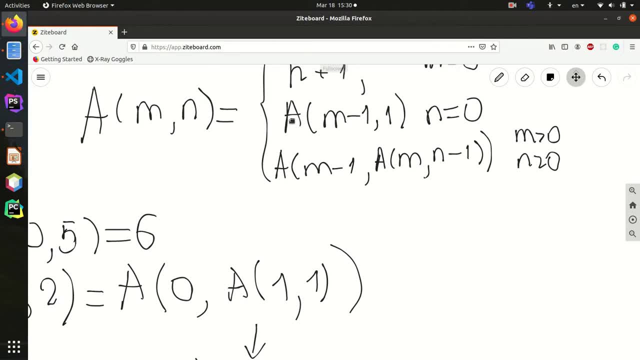 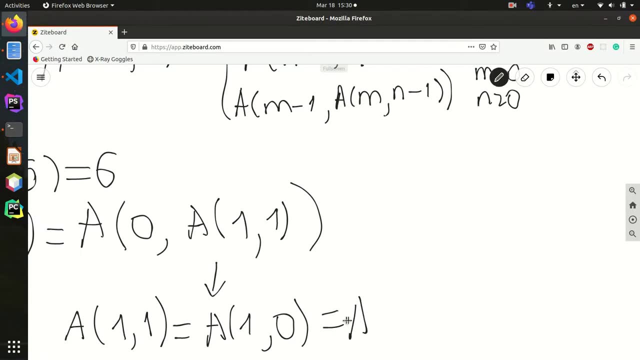 Okay, in this time, n is 0. If n is 0, I'm going to have this output, so it's going to equal to am minus 1, which is 1 minus 1, 0, and simply just 1.. 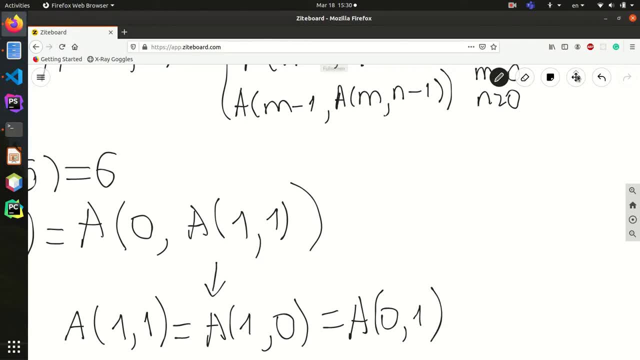 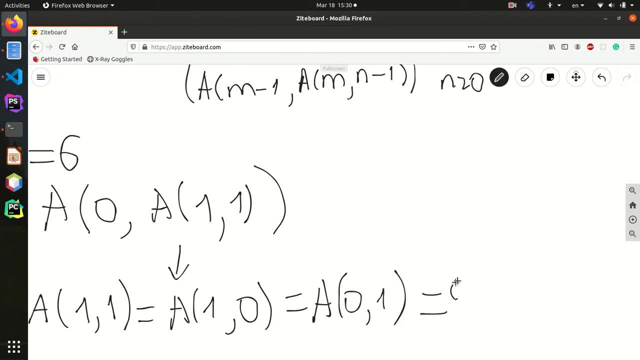 So, in this case, m is 0, and, as you know, if m is 0,, the output is going to be n plus 1, which is 1 plus 1, and it is 2.. So the output of m is 0.. 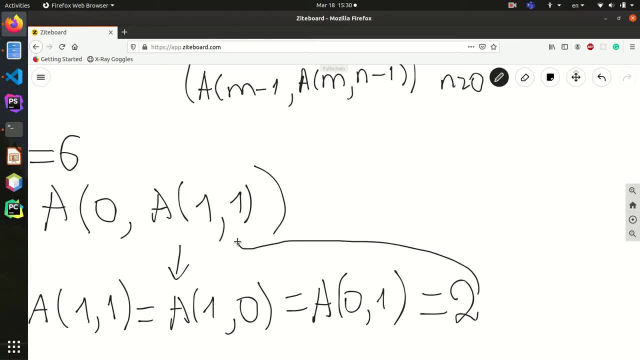 So the output of this function is going to be 2, so I'm going to come here and write 2 instead of a11, so it's going to equal to a02.. Okay, again I have 0, and I'm going to come here. m is 0. 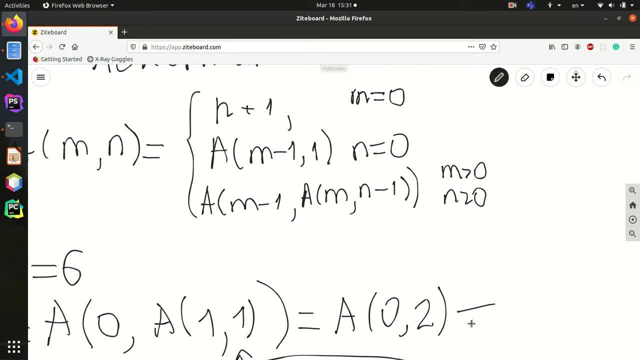 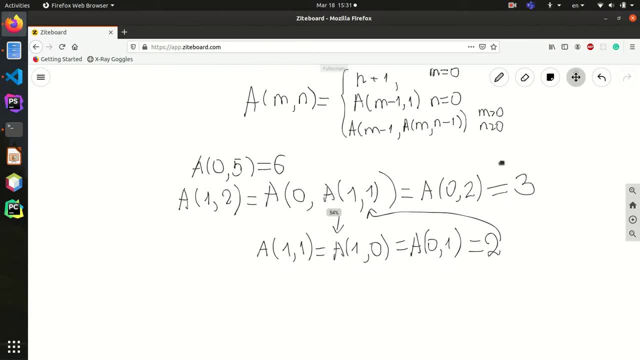 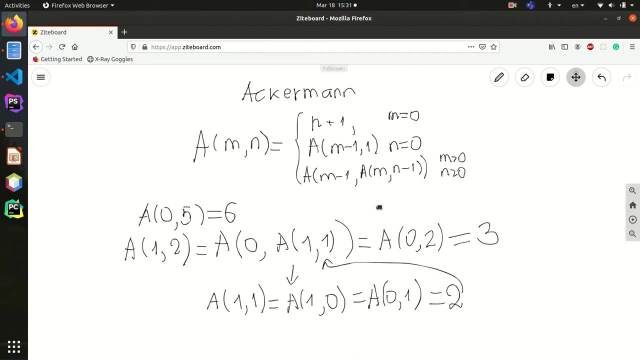 In case m is 0,, the output is n plus 1,, which is 2 plus 1, and 3.. Yeah, basically, this is it. This is how the function works. I hope it's clear for you, and I should mention that this function grows so fast, so you need to be careful. 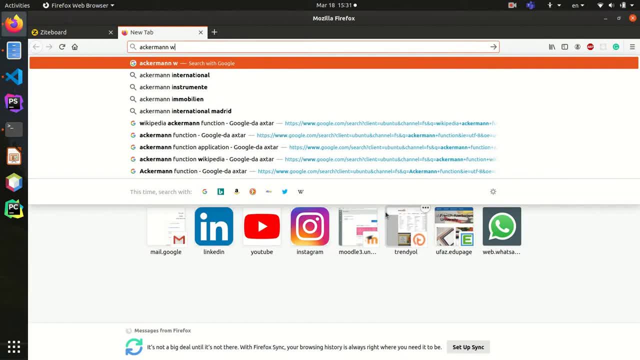 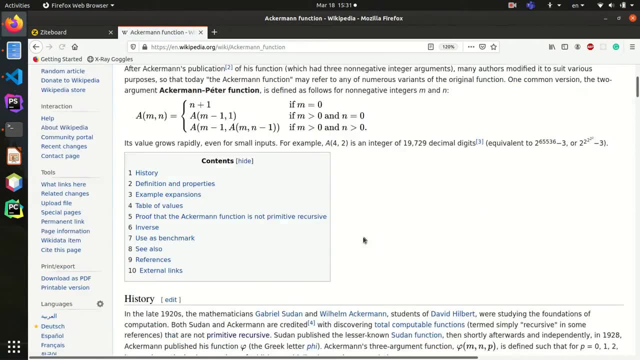 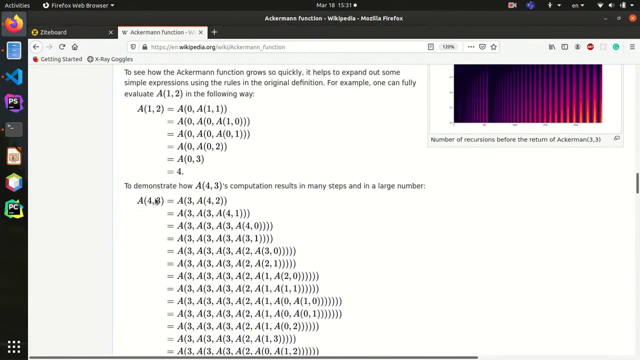 Let's check it with Wikipedia, Let's check the table with Wikipedia. So, as you see, when you have a function which is 4 and 3, it's going to calculate, it's going to call, say repeatedly, again and again. 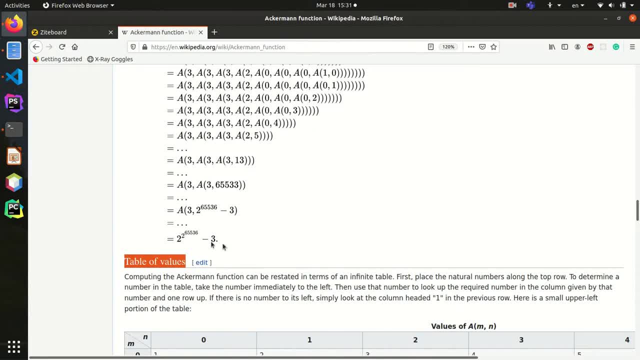 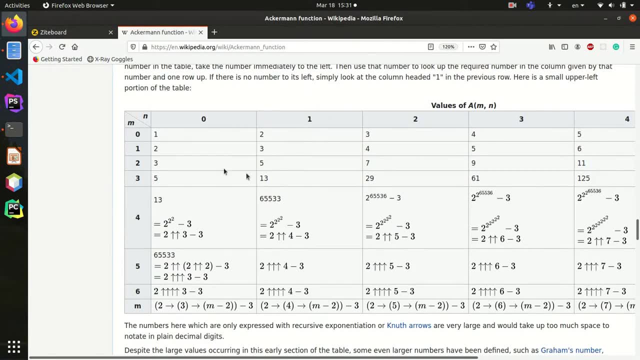 and then, as a result, at the end, you've got this output, which is quite big, So that's why your computer will not be able to calculate it. This is the table for values of mn. So, in case you have 0,, you've got 1.. 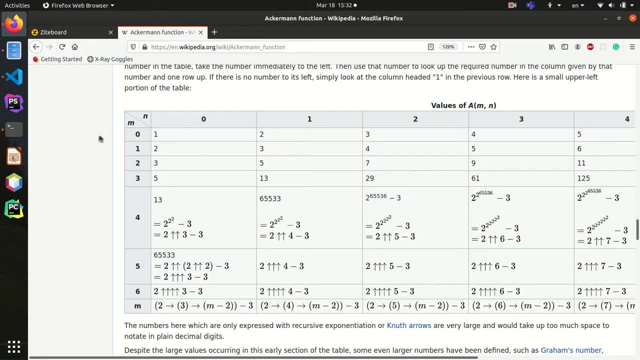 You have m0, n1,. you've got 2,. as it is clear for you, Whenever it is 0, the output is going to be n plus 1.. You have 3, 0,, 5,, 3,, 1,, 13,, 3,, 2,, 29,, etc. 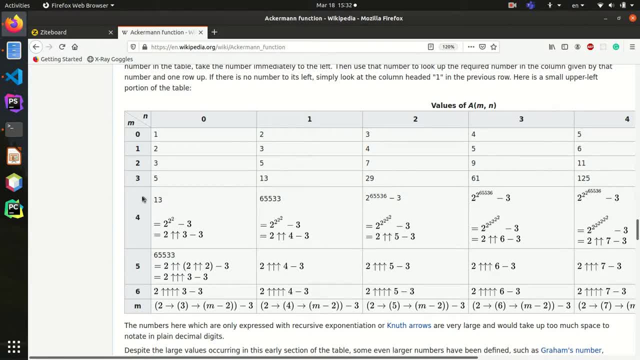 Everything is okay with 3 so far, But when you have 4,, you should be careful because, okay, you got the output. With 4, 0,, it's 13.. With 4, 1,, it is this number. 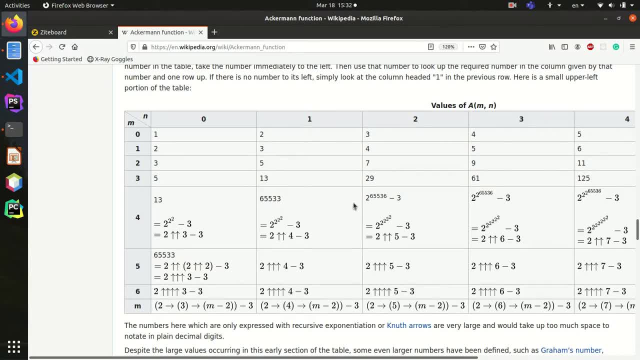 But with 4,, 2, it gets completed. So you have 4, 0,, 13,, 3,, 2,, 29,, etc. I think it's not going to calculate it either, But when you have 4,, 3, it gets more complicated. 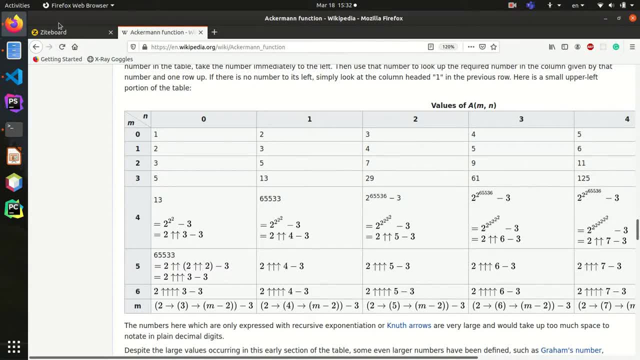 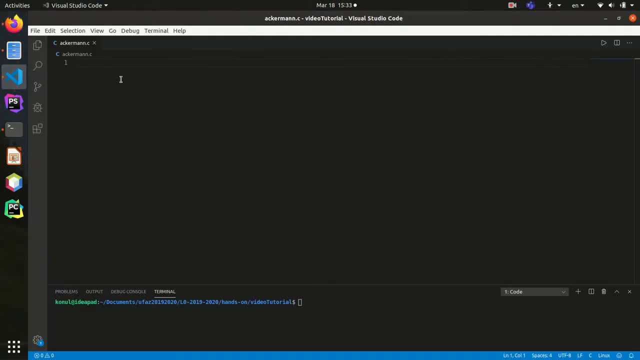 So your computer will not be able to calculate it. Now let's go and write this function in C. Let's see how it can be written. So, firstly, I'm going to include a standard input output header. That's what I need so far, because I'm going to use print. 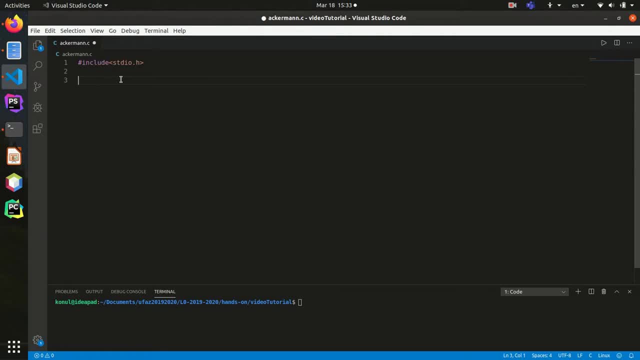 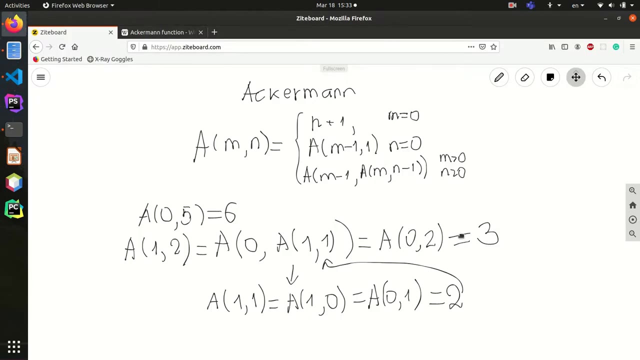 And I'm going to use scan function. So I have main function here. I just write it now. Now, above main, I'm going to write the prototype of Ackermann function. So Ackermann function returns me integer numbers. By the way, I should mention that m and n are non-negative values, okay. 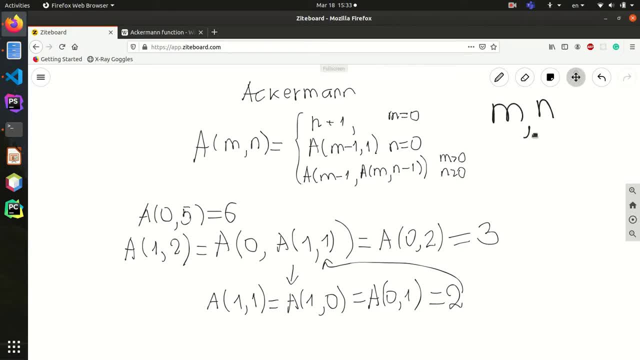 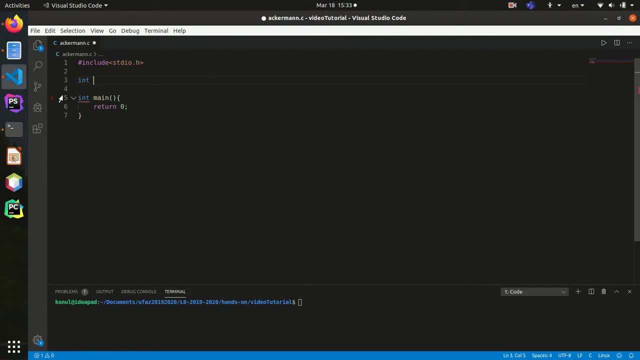 So I assume that's going to return me integer values. So I assume that's going to return me integer values. So I assume that's going to return me integer values- integer, and that's why I call its data type as integer and then I give it a name. I'm going to 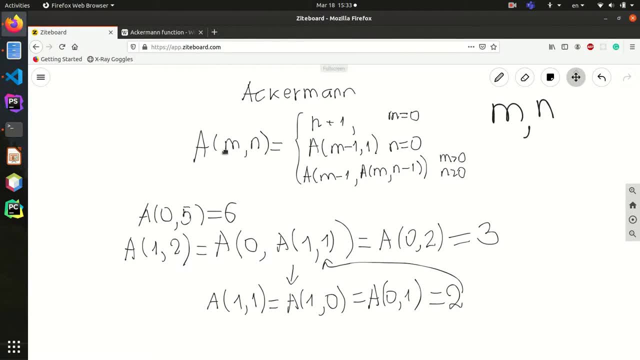 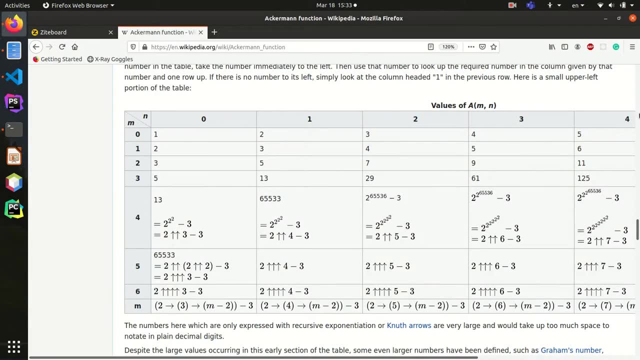 call it Ackerman. and Ackerman function takes two arguments, which is m and n, and they are also integer. I'm going to give only integer number 0,, 1,, 2, 3.. I can give only. I mean I'm going to check. 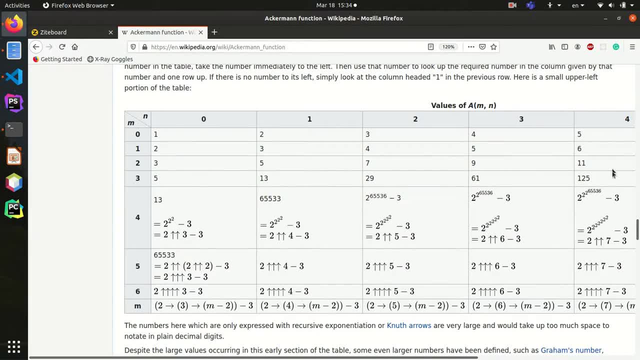 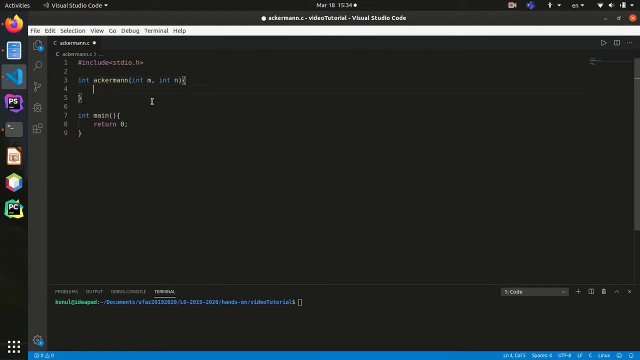 it with 3, 4, 3, 7, whatever, but I cannot check it with greater than 4 and 3 or 2.. So that's why I'm going to call this numbers integer as well: m and n. and now it's time to fill the inside of a. 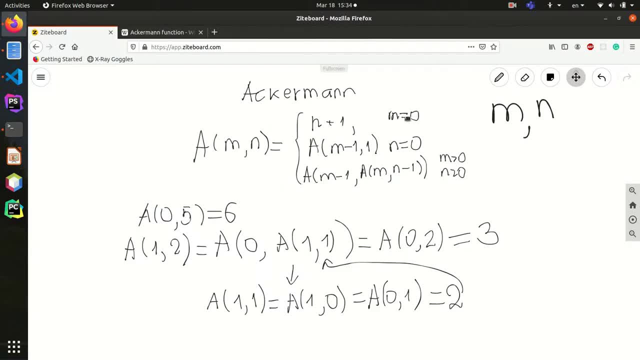 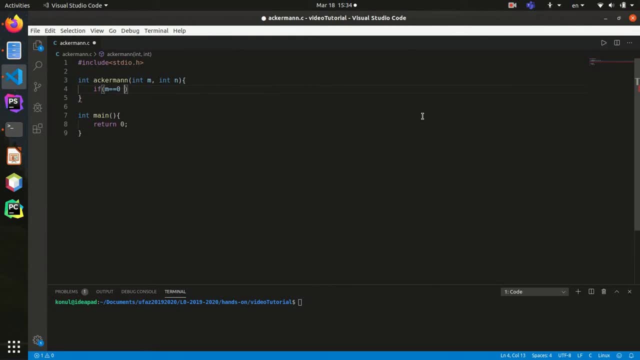 function. So I have three different conditions. First condition: if m is equal to 0, if m is equal to 0.. As I have mentioned, m and n should be non-negative numbers. that's why I'm going to write n is greater than 0. So in this case, the function is going to return n plus 1.. Return n plus 1.. 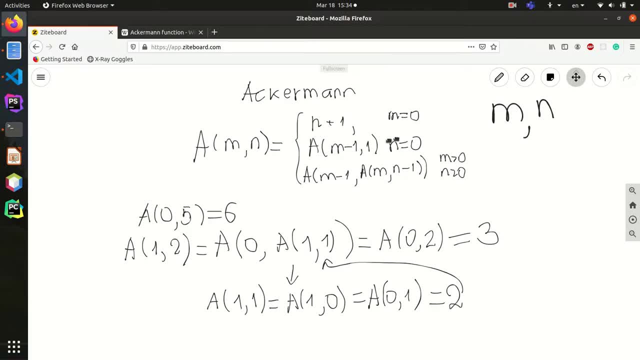 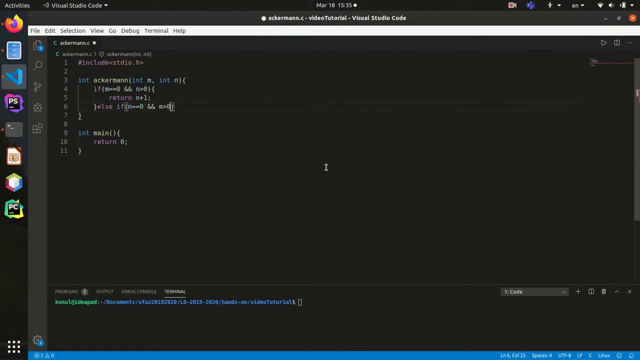 Okay, as if another condition which says n is equal to 0 and n is equal to 0 and m is greater than 0. In this case, return a m minus 1, 1.. Return, it's not a, so the function name is Ackerman, That's. 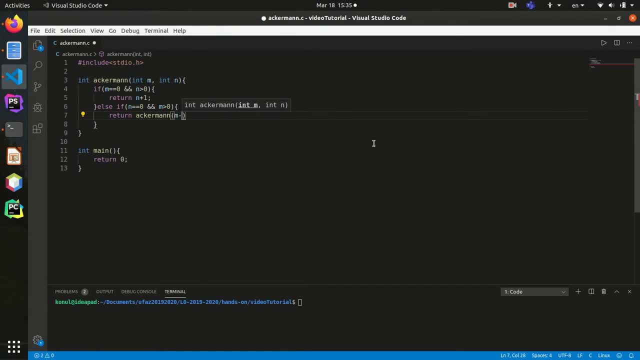 why I'm going to call it Ackerman m minus 1 and 1.. Else, if in case m is greater than 0 and n is greater than 0. In this case, returns us Ackerman. The result is now n-1, ackerman m-1.. Provided there's no 코로나. 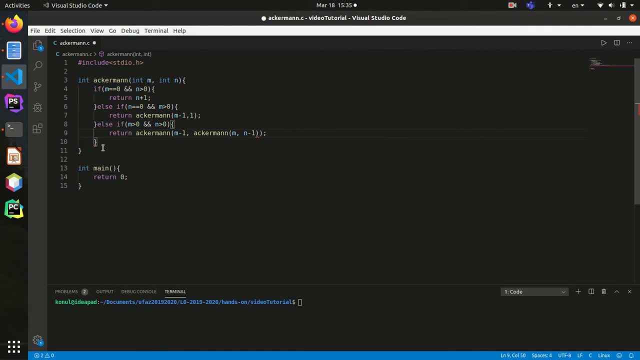 again one more Ackerman, m and n-1.. That's pretty easy, but uh, what I want to, what I want to say is that I'm going to write it. I'm going to write it just right after main function, but I'm going to declare. 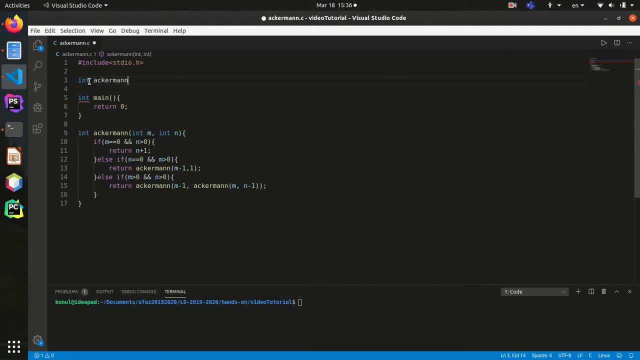 the prototype above main function. okay, so this is function prototype prototype. okay, the function is ready, we have filled the inside of a function and we can go ahead and do calculation and we can call it in main. so as the function takes two arguments, I'm going to have two different numbers here as well. well, 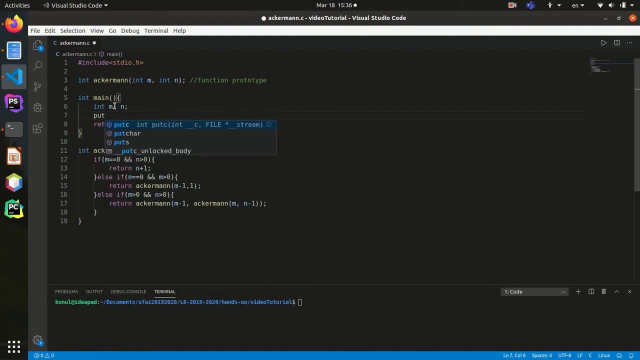 here variables here as well, and I'm going to ask user to enter numbers for M and N and after user enters, I'm going to save them in the address of those variables, which is M and N. after that I want to store the result of this function. 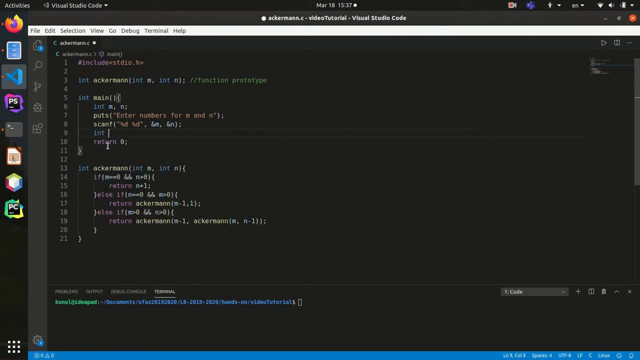 output of this function in a variable which is called result and I can write: result is equal to Ackerman. I'm going to pass arguments, parameters for this, which is M and N, and to see the result, I'm going to print it out. the result is percentage D, which is result. okay, 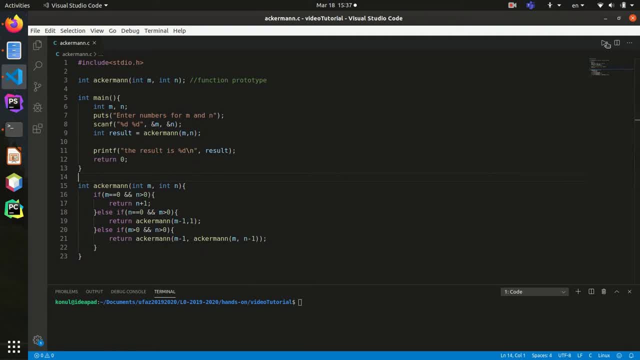 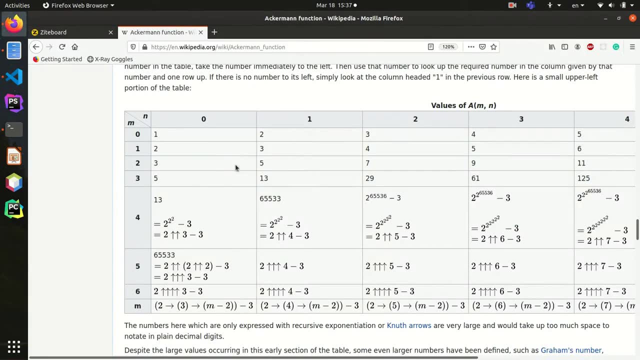 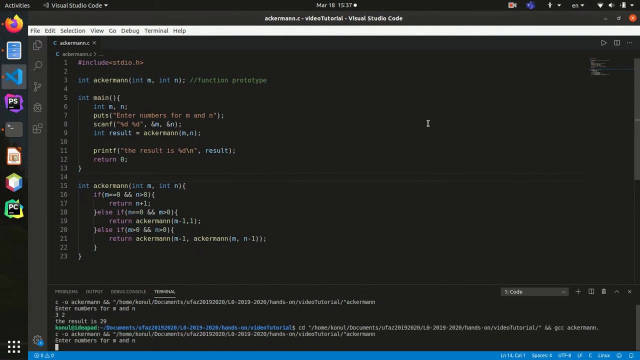 the function is ready, so we can go ahead and try to check if everything is okay. I seems everything is okay, and let's do it with this table. let's say that M is 3 and n is 2. 3 & 2. okay, the results is 29. good, now let's. 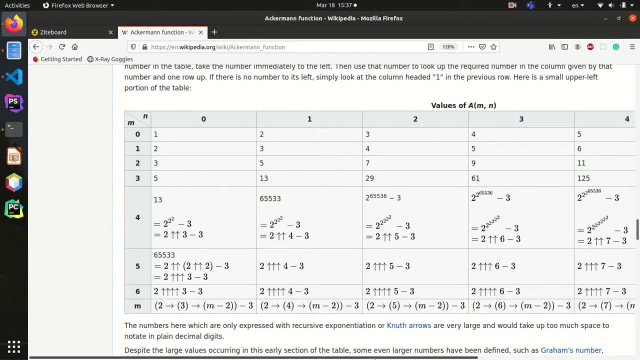 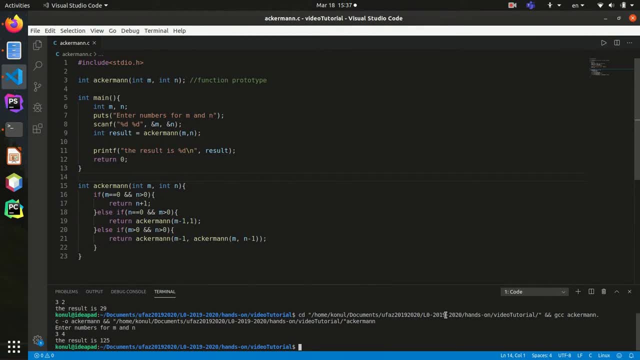 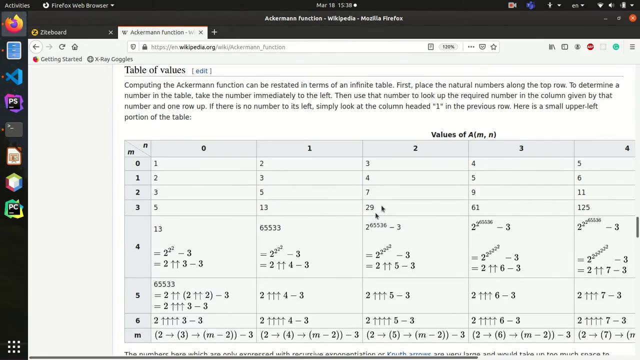 check it with 3 & 3 and 4. we can check it with 3 & 4. the result is good, we have 125, but the result it is good, we have 125, but but let's check it with 4 and 2 to see if we're gonna get the result or not. 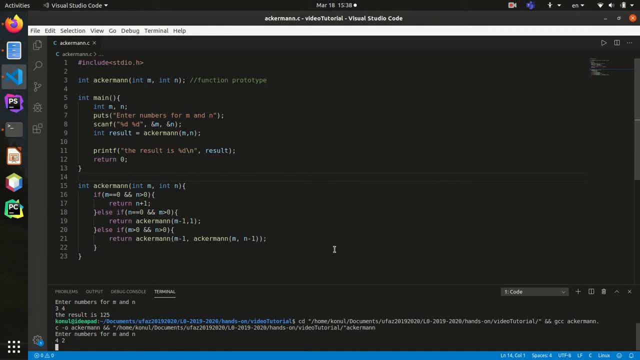 it's gonna be a big number. I don't know the computer can calculate it or not, but we will see the output. let me pause it for now. the numbers are: yeah, I think. yeah, it's a big number, so it couldn't completely calculate it either. yeah, basically, this is the all you need to know about. 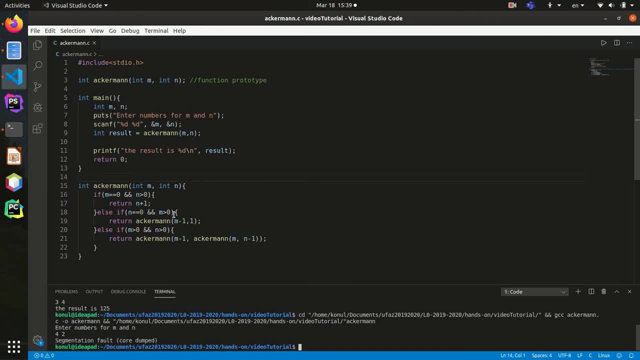 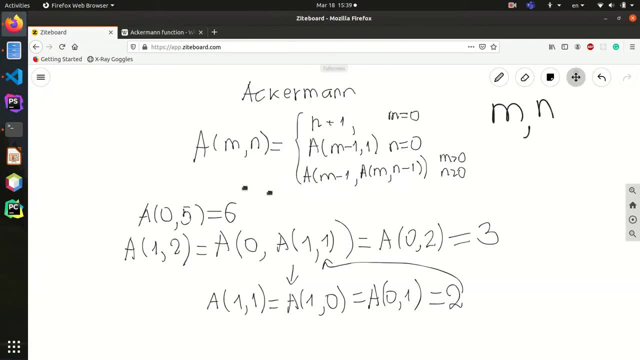 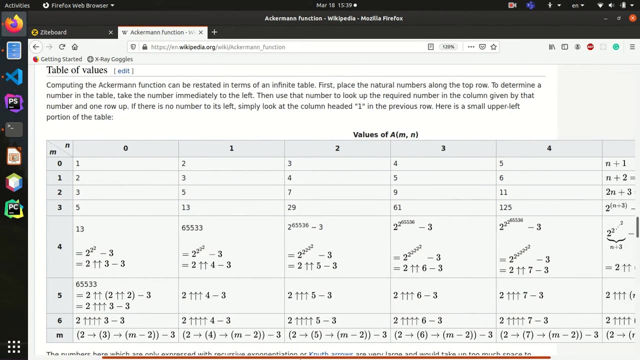 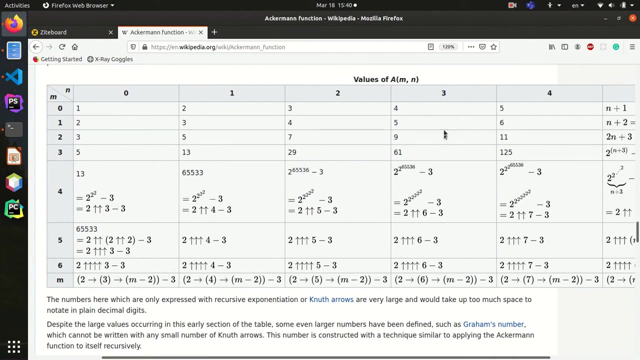 Ackermann function and how to write the function, how to convert it into C language and how it works, to understand how it works, etc. so if you feel uncomfortable about complete calculation of this function, go ahead and try to calculate the this function with those given numbers. for example. you can get by hand, you can calculate it. a3.